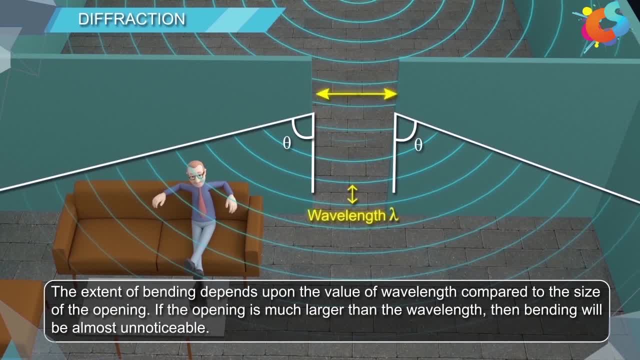 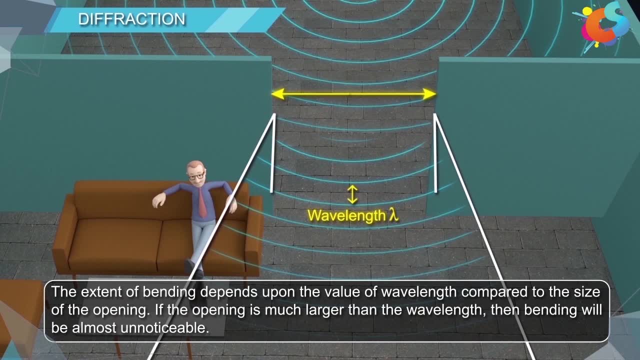 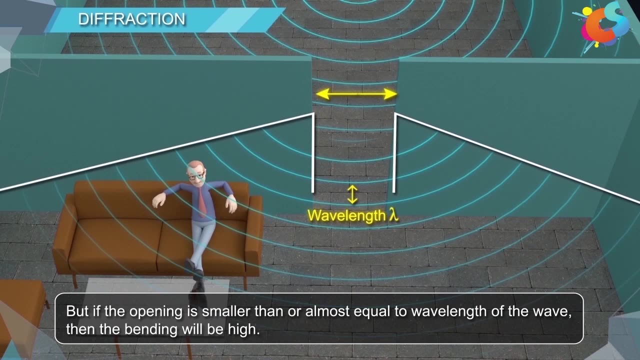 of wavelength compared to the size of the opening. If the opening is much larger than the wavelength, then the bending will be almost unnoticeable. But if the opening is smaller than the opening or almost equal to the wavelength of the wave, then the bending will be high. 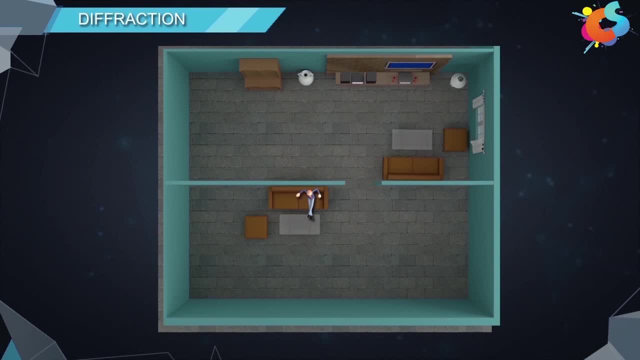 Now consider another situation where we have a light source instead of a music system. As we can see here, the light waves have illuminated only this part of the room. This means that the light waves did not bend to illuminate this region, This type of regions where a 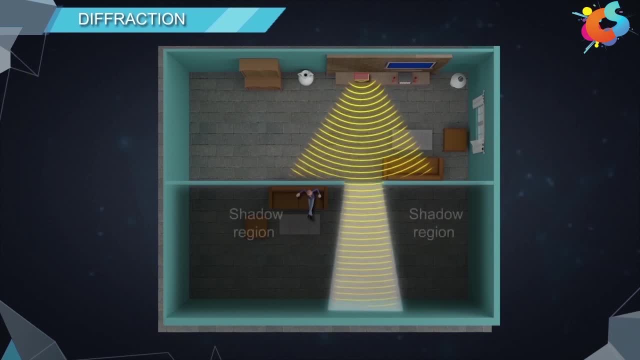 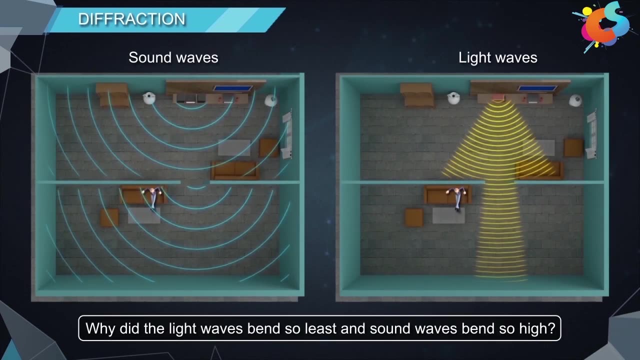 particular wave is unable to penetrate is called the shadow region. Now the question is: why did the light waves bend so least? Mhm, this is a match made for noise, and sound waves bend so high. The answer for this lies in the property of wave, which states that 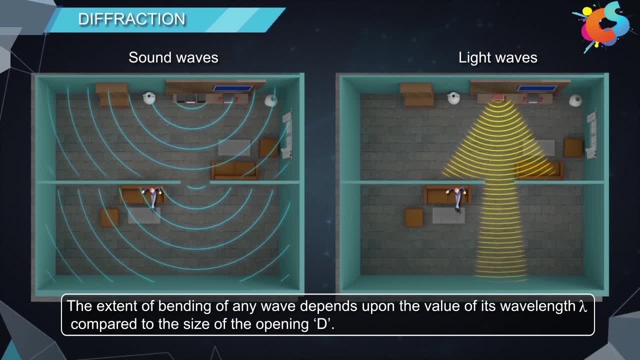 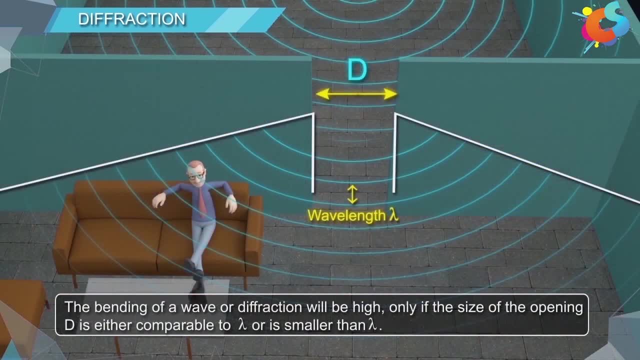 the extent of whether of any wave depends upon the value of its wavelength lambda compared to the size of opening D. The bending of a wave or any otra portion of any wave depends on its width instead of its eye or eye length. Then whose wavelength will mean when you bend or touch thegens that are contactw sucks more strongly, regardless of its length? Stopkach will display the Communist hydrogen everywhere. 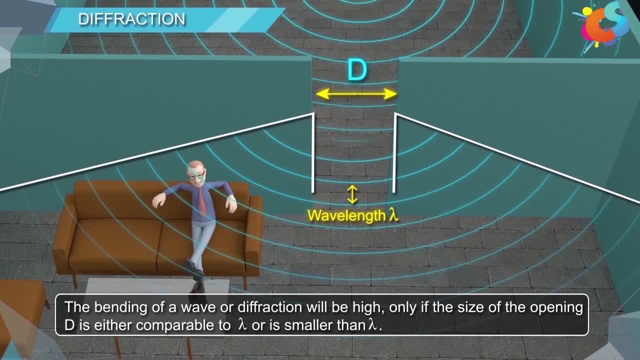 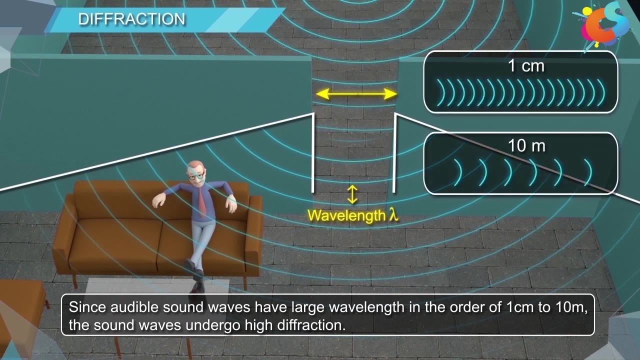 or diffraction will be high only if the size of the opening D is either comparable to lambda or is smaller than lambda. Since the audible sound waves have large wavelength, in the order of 1 centimeter to 10 meter. the sound waves undergo high diffraction. However, the wavelengths of visible light is 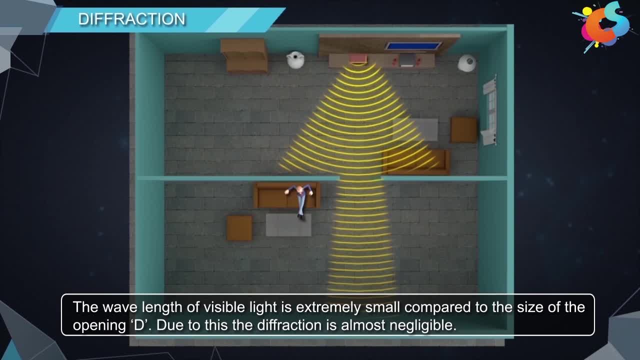 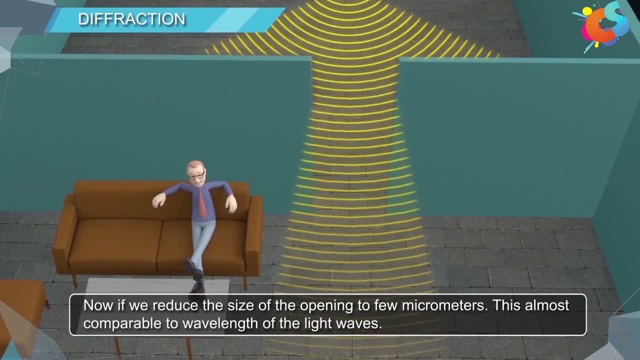 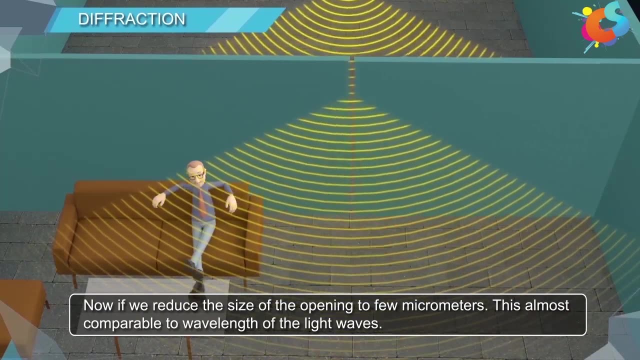 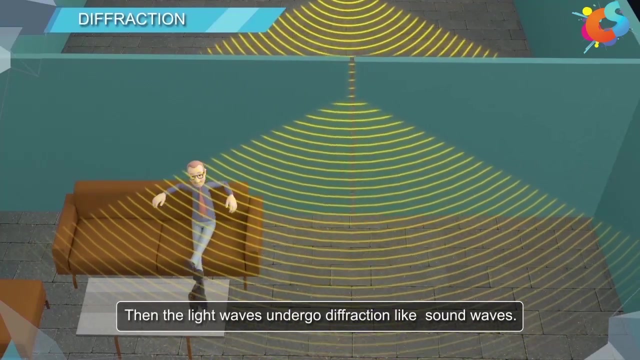 extremely small compared to the size of the opening D. Due to this, the diffraction is almost negligible. Now, if we reduce the size of the opening D- few micrometers, which is almost comparable to wavelength of the light waves- then the light waves undergo diffraction like sound waves. 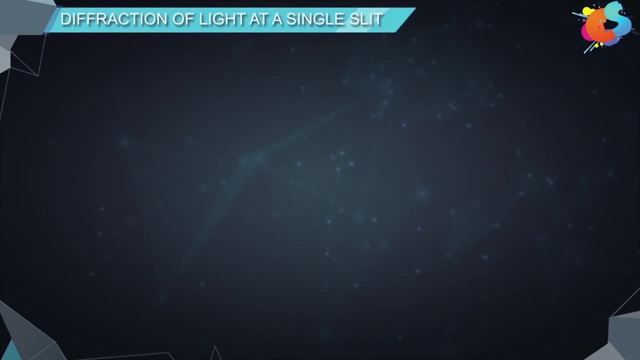 Fraunhofer's diffraction at a single slit. When a monochromatic light wave is allowed to operate, this diffraction is one of the most difficult to perform. When a monochromatic light wave is allowed to operate, this diffraction is one of the most difficult to perform. 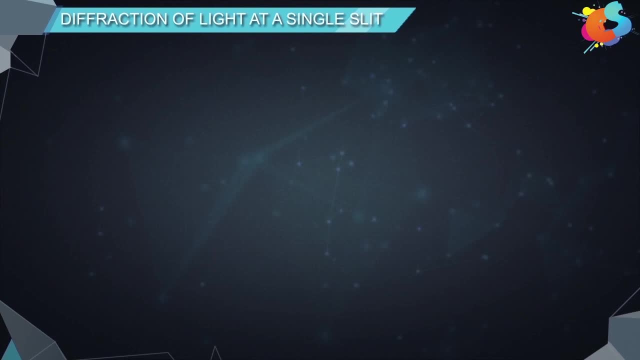 to fall on a tiny opening with size in few micrometers. the light undergoes diffraction. Now, if we place a screen in front of the opening, alternate dark and bright pattern is formed on the screen. Now let us discuss about the diffraction pattern formed by a monochromatic 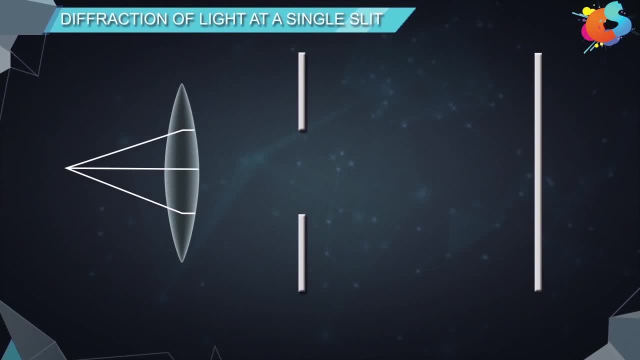 light source. Consider a plane wavefront xy of wavelength lambda incident on a narrow slit ab of width a. According to Huygens principle, every point on the wavefront at the slit will become source of secondary wavelets. Waves of same amplitude are emitted from these points. 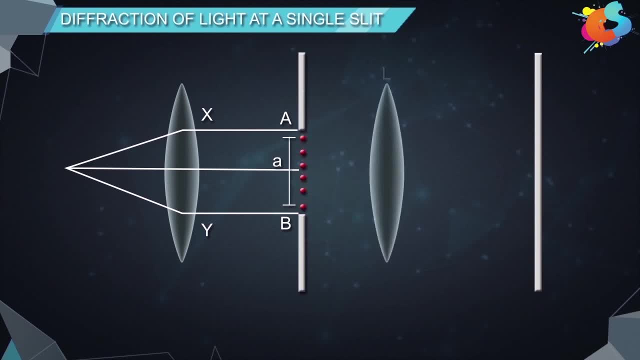 in all directions. With the help of a convex lens L, all these slits will become the source of secondary wavelets. With the help of a convex lens L, all these slits will become the source of secondary wavelets. waves are focused onto a screen placed at a distance d from the slit. 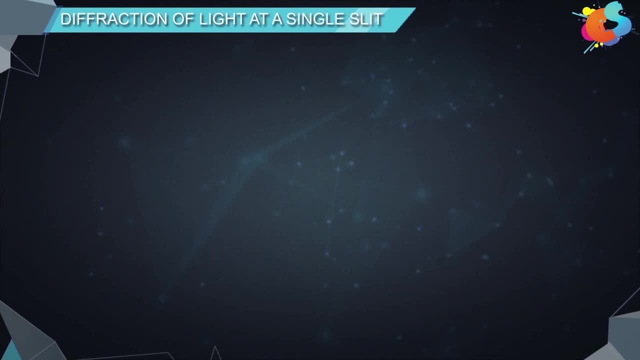 A diffraction pattern is obtained on the screen and the pattern consists of alternate bright and dark bands of decreasing intensity on either side of the central maximum. Now let us calculate what causes these bands. Now consider a point O on the screen which lies on the perpendicular bisector of the slit, The wavelets that fall on the lens L1. 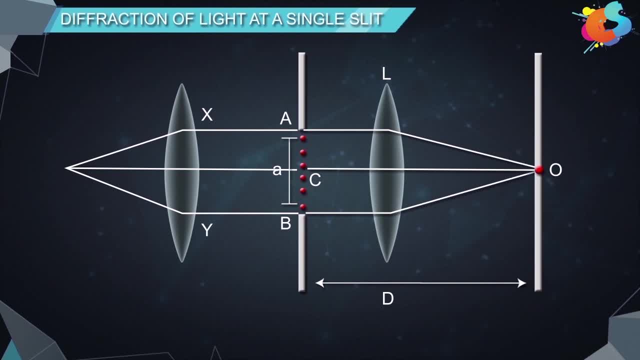 parallel to CO, converge on point O. since the waves from these points travel equal distances to reach point O, The phase difference between them will be zero. The waves superpose with each other and produce maximum intensity at O. This point O becomes the location of central bright. 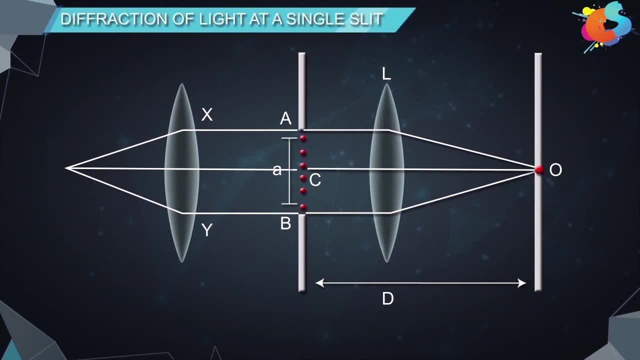 fringe. Now consider an arbitrary point P on the screen. All the secondary waves from the slit AB make an angle theta with CO and reach the point P. The intensity at point P depends on the path difference between the waves. Now let us draw a perpendicular AN from the point A to this ray diffracted from B. Now the distance. 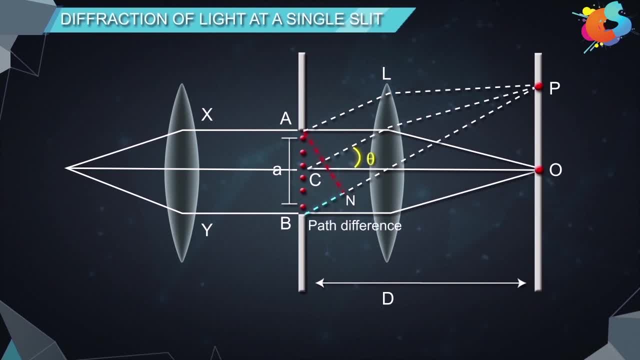 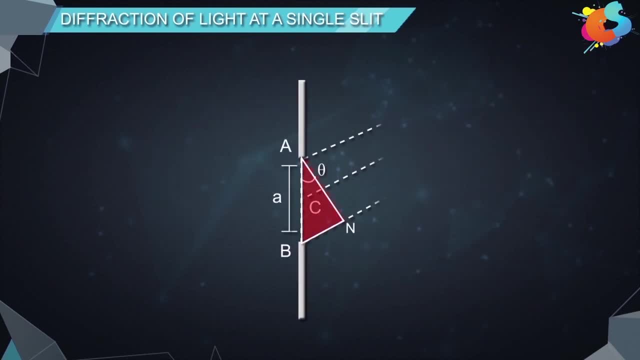 BN gives the path difference between the secondary waves from A and B reaching point P From triangle ANB. BN by AB is equal to sin theta and BN is equal to AB sin theta, Since AB is the slit width, which is equal to A, and BN is the path difference. 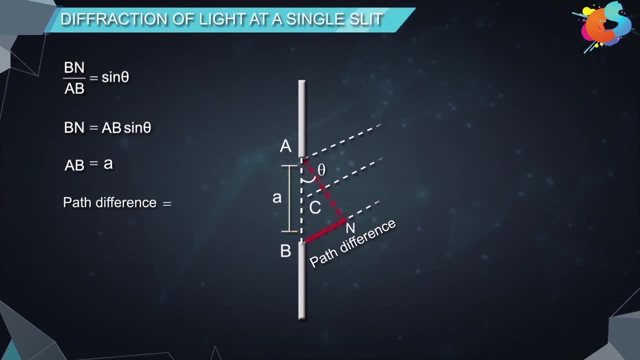 Therefore, the path difference is equal to A and BN. is the path difference equal to A sine theta? Now case 1, if the path difference between the waves is equal to lambda, To analyze this condition, let us divide the whole wave front. 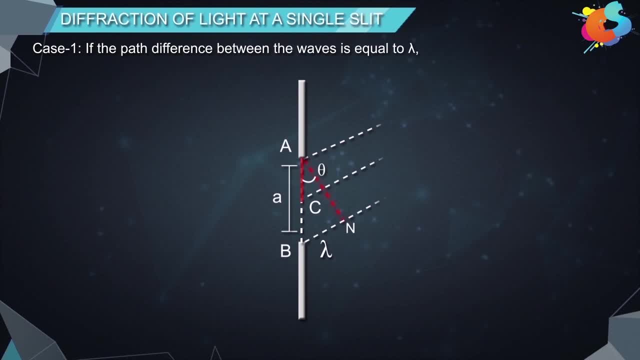 AB into two equal halves, AC and CB. Since the path difference between the secondary waves from A and B is lambda, the path difference between the secondary waves from A and C reaching P will be lambda by 2.. Due to path difference of lambda by 2, these two waves will interfere. 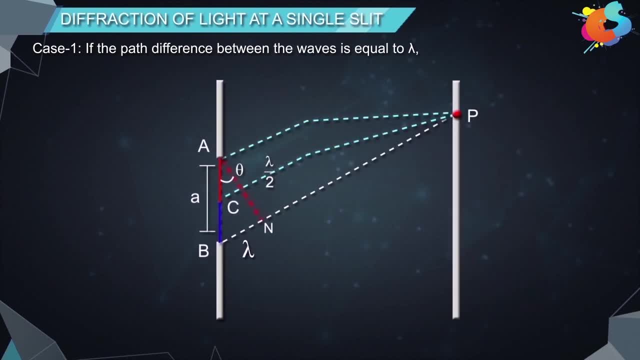 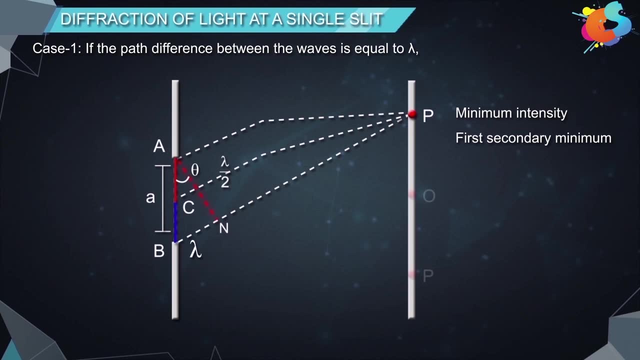 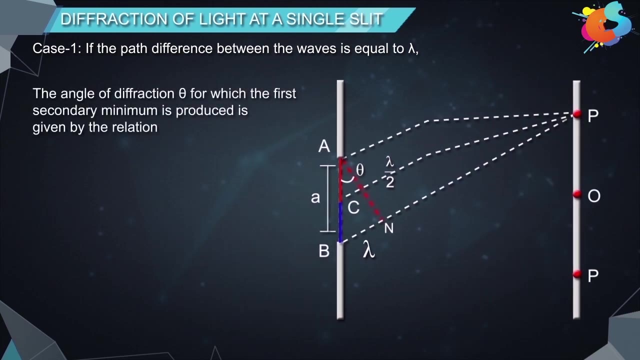 destructively at point P. Overall, point P will be of minimum intensity and it is called first secondary minimum and it is formed on either side of the central maximum. The angle of diffraction theta for which the first secondary minimum is produced is given by the relation A: sine theta is equal to lambda or sine theta is equal to lambda. 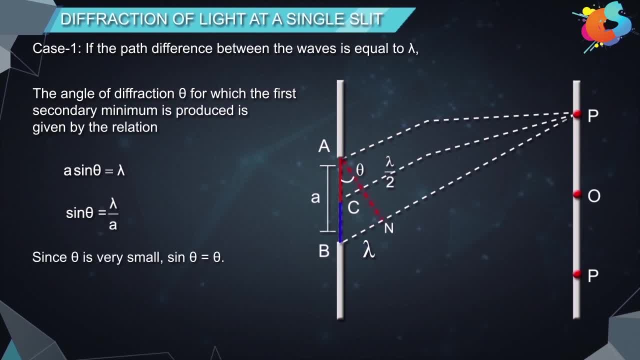 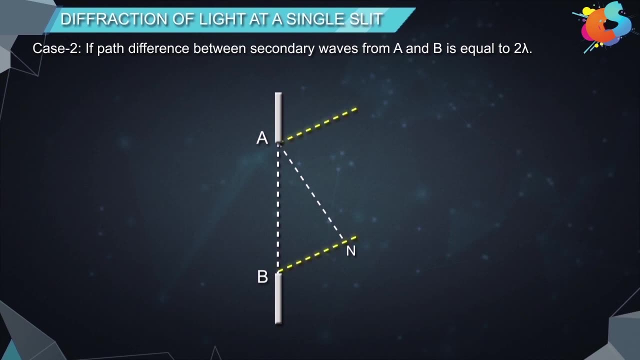 divided by A. Since theta is very small, sine theta is approximately taken as theta. Therefore, theta is equal to lambda by A If the path difference between secondary waves from A and B is equal to 2 lambda. In this case the wave front is equal to lambda by 2.. So 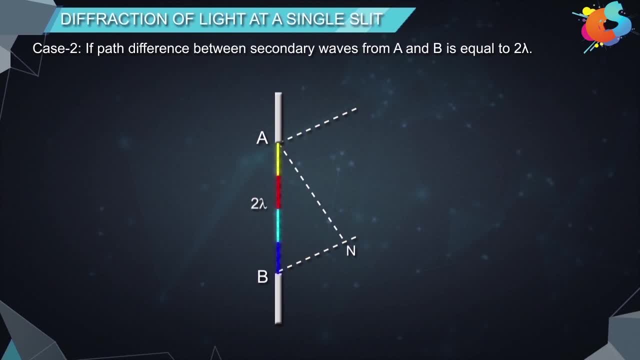 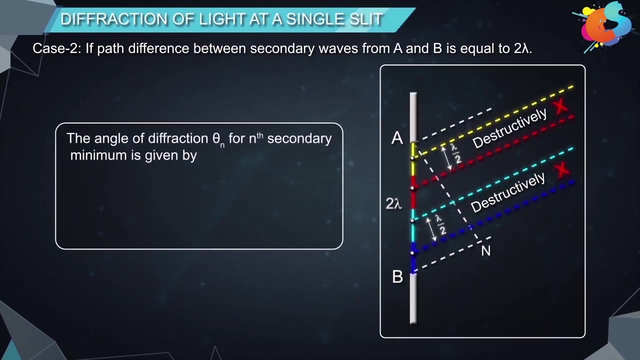 front AB can be divided into four equal parts. Now every point in a part will have a point in its adjacent part for which the path difference is 2, lambda by 4 or lambda by 2. Hence all these waves will interfere destructively In general the angle of diffraction theta. 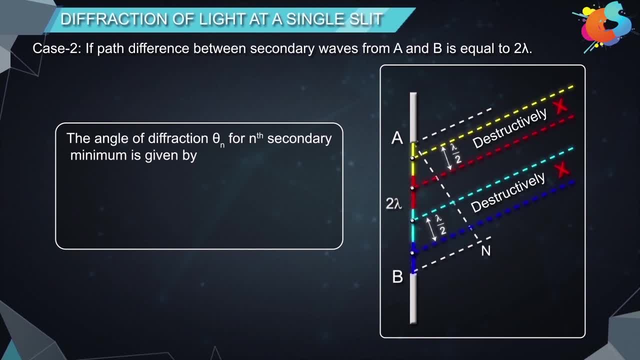 n for nth secondary minimum is given by theta n for nth secondary minimum. A sine theta n is equal to n lambda, where n is equal to 1,, 2,, 3,, 4 and so on. Now let us find the positions of secondary maxima. 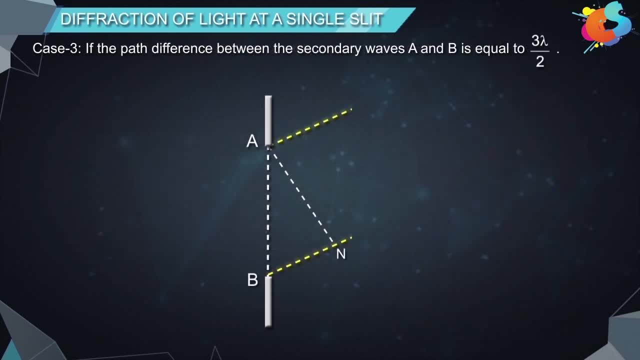 If the path difference between the secondary waves A and B is equal to 3 lambda by 2. In this case, the wave front AB can be divided into three equal parts. The path difference between the corresponding points of the first two parts will be equal to lambda. 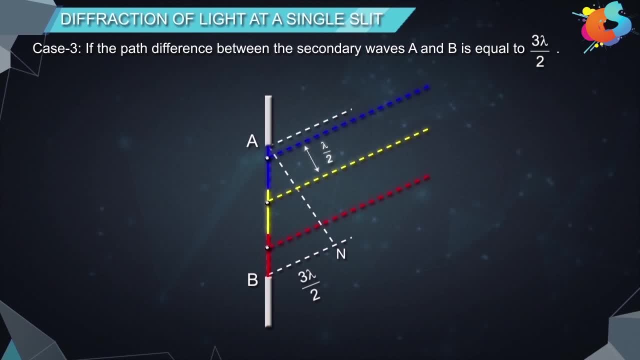 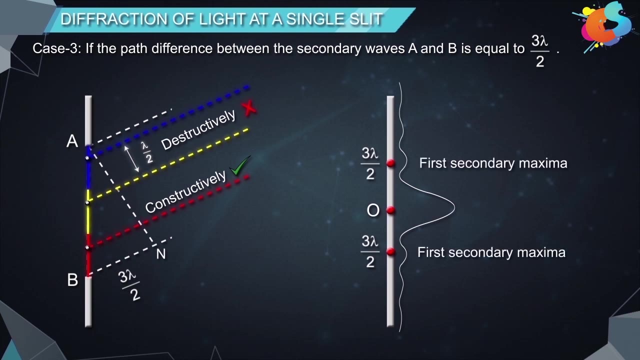 by 2. Therefore they will interfere destructively. However, the wavelets from the third unused part will interfere constructively at point P to produce a weak first secondary maxima. Similarly second secondary maxima will be formed on the screen where the path difference. 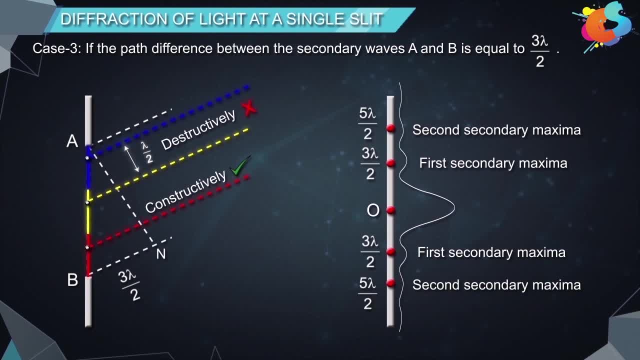 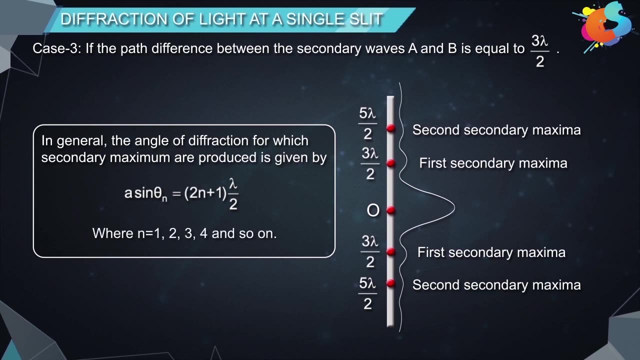 is equal to 5 lambda by 2.. In general, the angle of diffraction for which the secondary maxima are produced is given by A sine theta, n is equal to 2n plus 1 lambda by 2, where n is equal to 1,, 2,, 3,, 4 and so on. Now let us look at the width of the central. 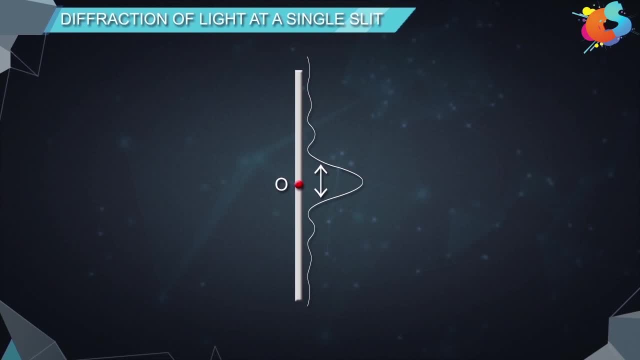 maximum. The linear width of the central maximum is the distance between the first secondary minimum on either sides of the central maximum. at O. Linear width of central maximum is given by: W is equal to 2 lambda D divided by A. Here D is the. 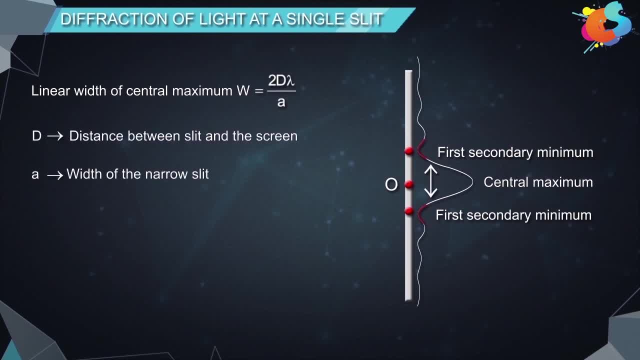 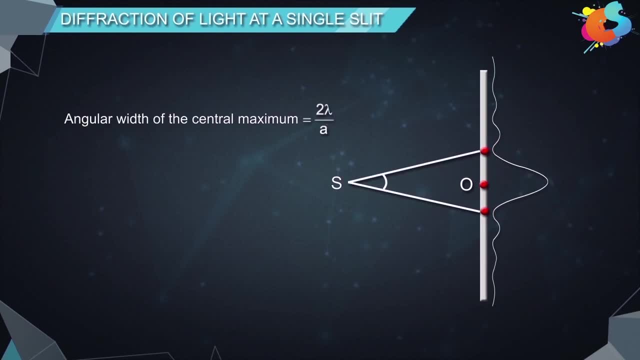 distance of the screen from the slit. A is the width of the narrow slit and lambda is the wavelength of the light. Angular width of the central maximum is given by. omega is equal to 2 lambda D divided by A, And the units of angular width is radian. Figures here shows the Intensity of: 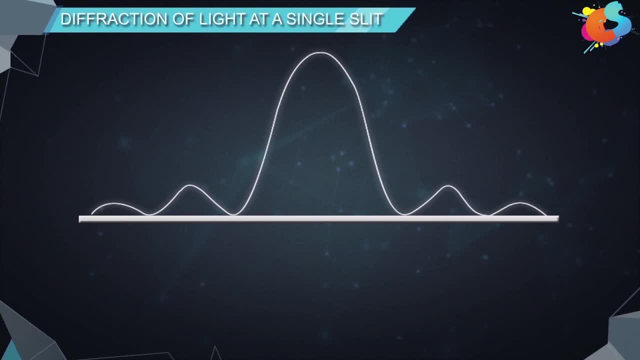 diffraction pattern for single slit for various angular positions sine theta. The pattern has central bright maximum formed at point O. The angular positions of various secondary minima are sine theta. is equal to: plus lambda by A, minus lambda divided by A. minus lambda divided by A.